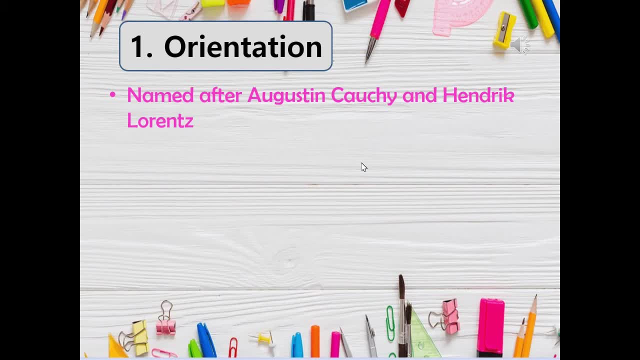 It is a family of continuous probability distributions which resemble the normal distribution family of curves. While the resemblance is there, it has a taller peak than a normal and, unlike the normal distribution, its fat tails decay much more slowly. The Cauchy Distribution is well known for the fact that its expected values and other 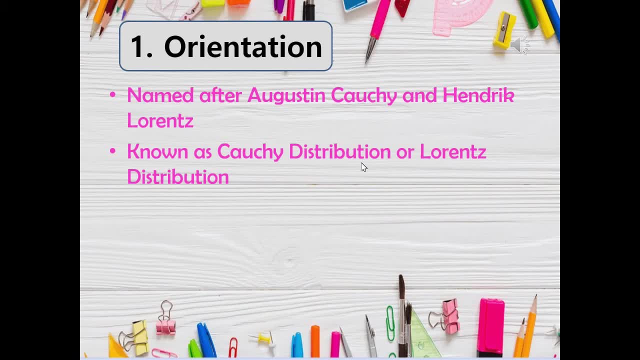 moments do not exist. The median and mode do exist and for the Cauchy they are equal Together. they tell you where the line of symmetry is. However, the central limit theorem doesn't work for the limiting distribution of the mean. 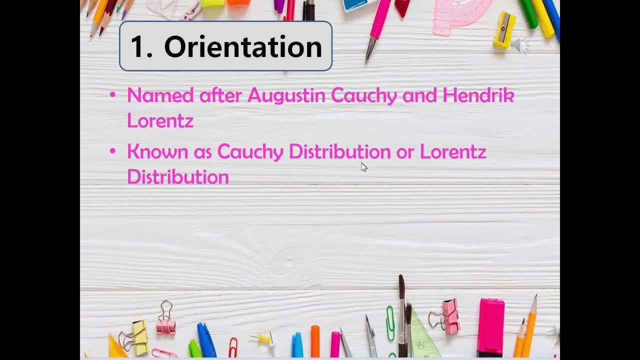 In sum, this distribution behaves so abnormally it's sometimes considered the Hannibal Lecter of distributions. On the other hand, this distribution also has its significance. It is used to describe resonance behavior. It is a popular distribution for robustness studies. 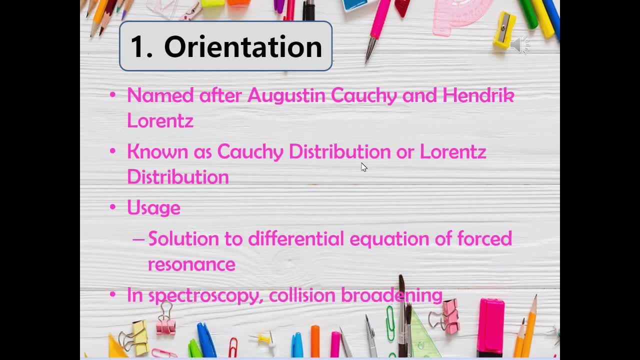 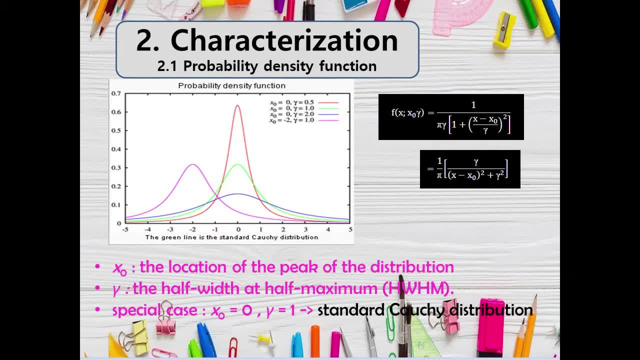 In quantum mechanics. it models the distribution of energy of an unstable state and collision broadening in spectra. Cauchy distribution: The Cauchy distribution is a family of continuous probability distributions which resemble the normal distribution family of curves. It has two main parts: a scale parameter and a location parameter. Now let's 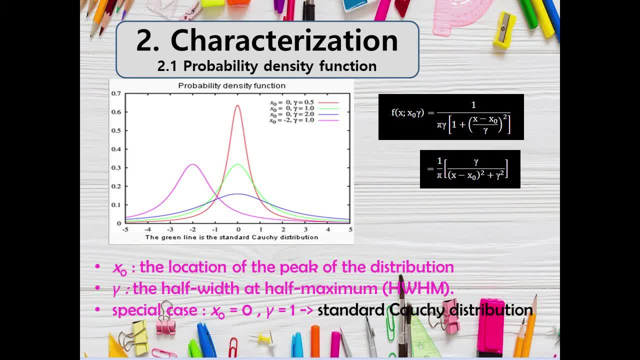 differentiate the two. First, we have the location parameter exo. It tells us where the peak is, While the scale parameter is half the width of the PDF at half the maximum height, And we'll gonna know how does each looks like later on In other. 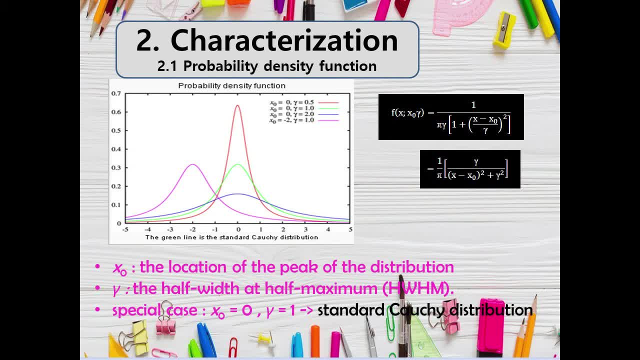 words. the location parameter exo shifts the graph along the x-axis and the scale parameter lamba results in either shorter or taller graph. Now let's take a look on the graph. Does the graph has different curves? Yes, it has. How about the? 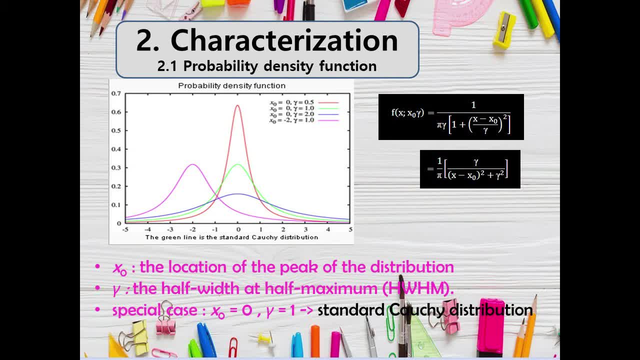 colors. It has what colors It has? red, green, blue and pink. Now let's examine the location parameter and the scale parameter. Let's start with the location parameter exo. Remember that the location parameter tells you where the peak is. Now let's have first the red curve. For the red curve, the peak is a. 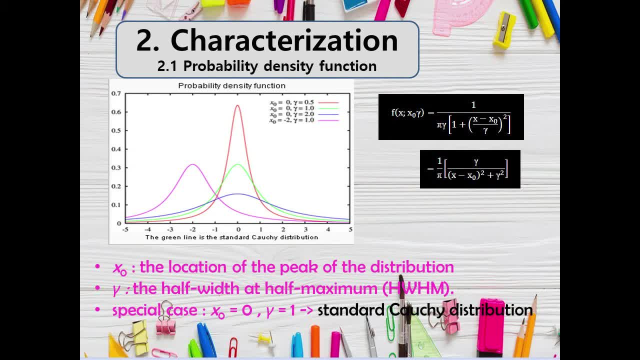 line or adjacent to zero. and it goes the same with the green and blue. How about the pink? For the pink, the peak of the pink curve is aligned to negative 2. That's why the value of the pink curve is negative. 2. For the location parameter: 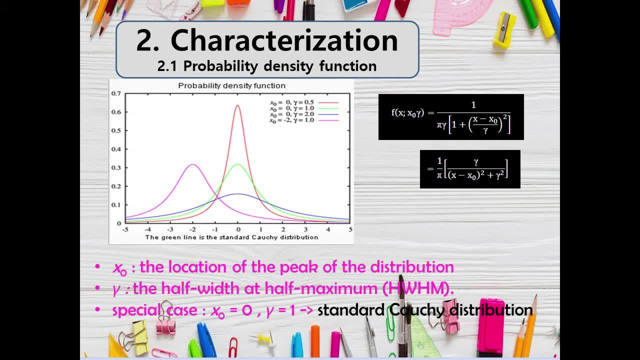 Now we're done there with the location parameter. let's have the scale parameter. Remember that the scale parameters have to be the of the PDF. so we're talking about the width of the PDF, So we're talking about the objetive value. this is F. Now we're done with the location Parameter. let's jump to the next picture. memory Localize is one point critical: that this can be just as broad as the larger size value, as wide as the drop-down speed value and similar quality values can be given by凹. and as the order track is half the position. 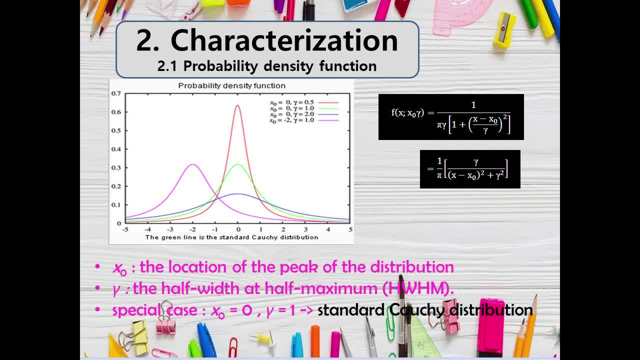 with the red curve. for the red curve it's 0.5, for the green it's 1, blue is 2, pink is 1. let's examine the values of the scale parameter. what is the smallest value of the scale parameter, or which curve has? 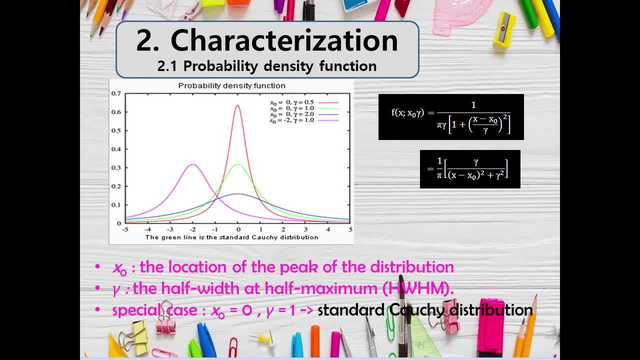 the smallest value of the scale parameter, it's the red curve, which is 0.5. it goes the same with the concept that the smaller the scale parameter, the taller and thinner the curve is. is it true that the red curve has the tallest and the thinnest curve? yes, it is. that's why it's true with that concept that the 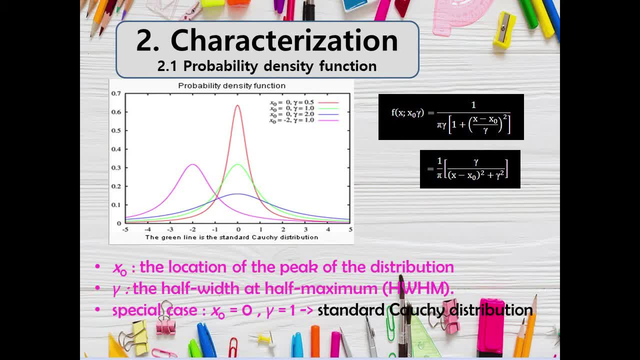 smaller the scale parameter. the smaller the value of the scale parameter, the taller and thinner the curve is. now let's take a look with the green curve. for the green curve, the location parameter is 0, while for the scale parameter it's 1, and it applies a special case of the standard Cauchy. 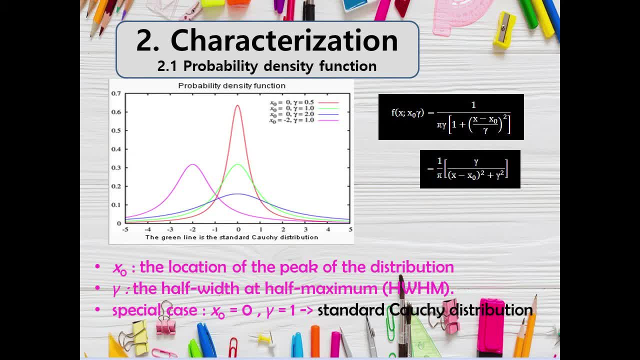 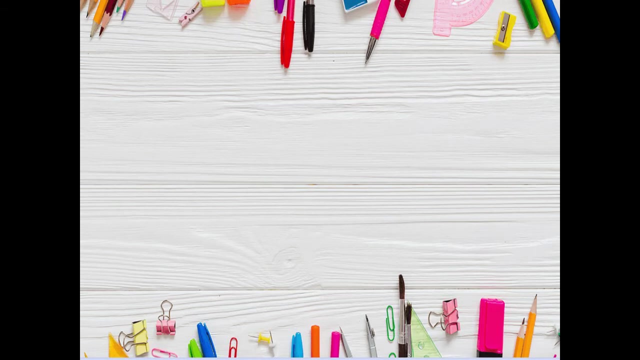 distribution that says XO, or the location parameter, which is 0, and the Lamba, which is the scale parameter, 1 is the standard Cauchy distribution. for the formula for PDF you can see it here: it's 1 over PI, Lamba over X, minus XO squared plus Lamba squared. the Cauchy distributions group is called the Cauchy Distribution Group. 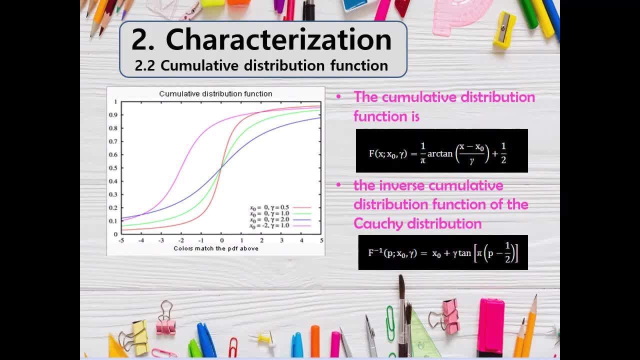 I'll be discussing to you each characterization and the same time I'll be discussing as well the probability density functions. but before I explain probability density density functions, I would like to expound first with the word cumulative distributions, as we all know that this one is used to calculate the area under the curve to the left. 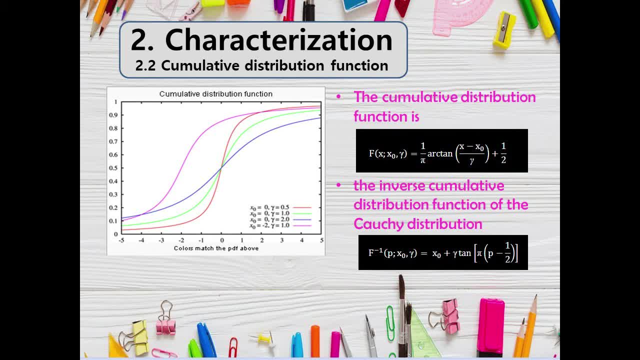 from a point of interest. it is used to evaluate the accumulated probability for continuous probability distributions, and that is the area under the core, which is equal to one, and the difference between cumulative distributions and the probability density functions, or the PDF is. it describes the shape of the 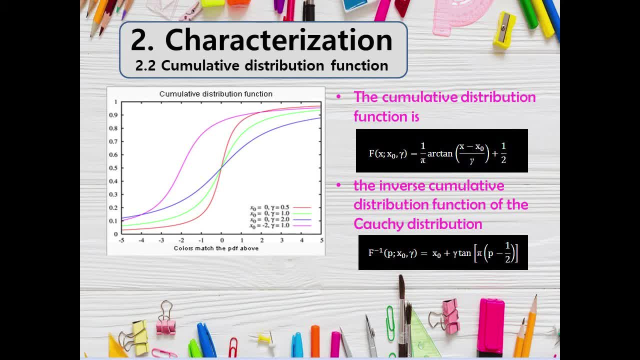 distributions. I have here some examples like the uniform distributions, exponential distributions or the normal distributions. I'm gonna go first for the uniform distributions, which is equal to f of X and that is equal to 1 over B minus a. and if I'm gonna describe the probability density functions, it looks 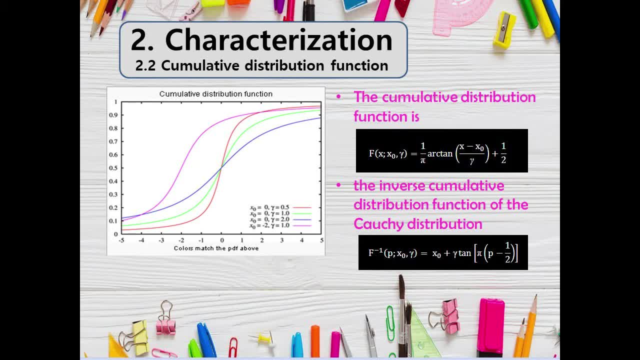 like a rectangle here for the uniform distributions we're in. the highest, or the highest point is the function of X, and below that will be at the distance between a and B, wherein X is in the middle. and what is this? if I'm gonna compute the cumulative distribution, 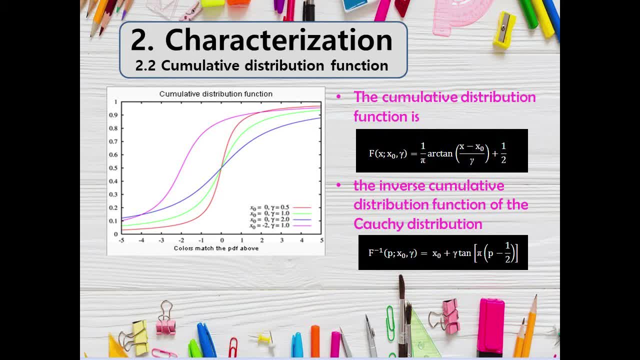 functions. the formula will be the area to the left of X. physically, the area will just be B times H, or that is equal to X minus a times F and the function of a and a of x, and that is an equal to x minus a times 1 over b minus a, or it is equal to the probability. 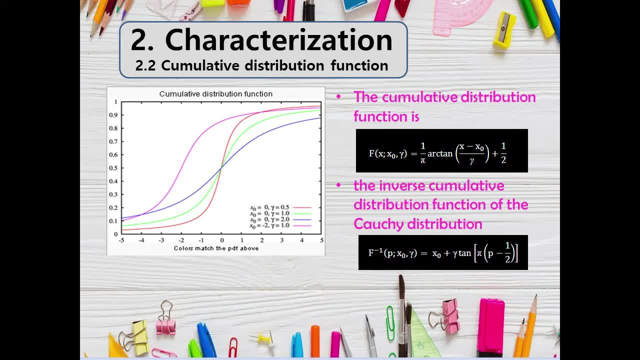 of the capital letter x less than or equal to some number, x, which is equal to x minus a over b minus a. Okay, moving forward. Okay, moving forward here. for what is this? Okay for the exponential distributions. I could say that if we're gonna drop the exponential 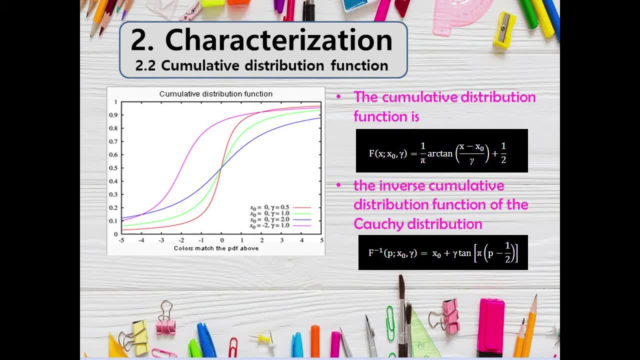 functions, the highest point will be the y intercept. that's the y intercept, and then for the exponential distributions, I could say that or equal to lambda, symbol lambda and it decreases all the time going down, and that is the probability density function formula- is equal to the function of X. 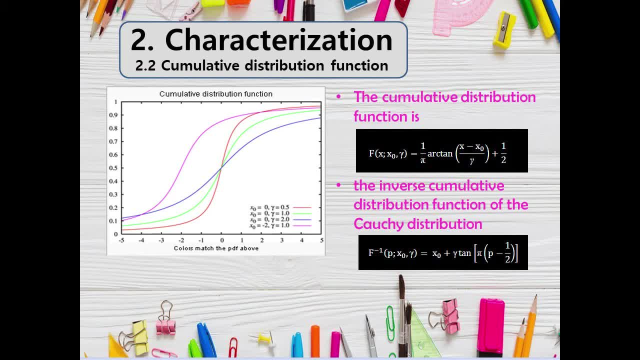 which is equal to lambda e raised to the power of negative lambda times X, where in lambda is just equal to 1 over the mean. okay, and to compute, since the probability density functions is the area to the right, the formula will be 1 minus quantity, 1 minus e raised to the power negative lambda X, simplifying that. 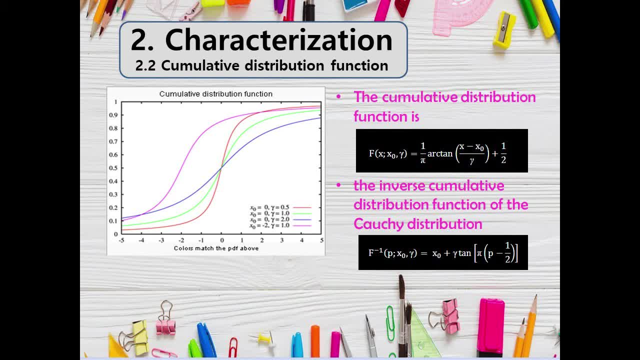 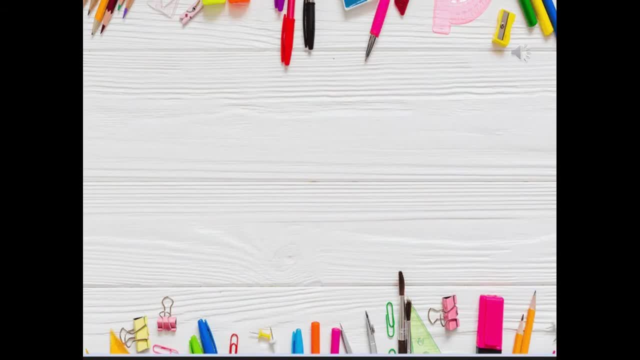 one, the area will just be equal to e raised to the power negative lambda X. thank you so much. the Cauchy distribution is an example of a distribution which has no mean variance or higher moments defined. its mode and median are well defined and are equal X sub 0 when you and V are two independent normally. 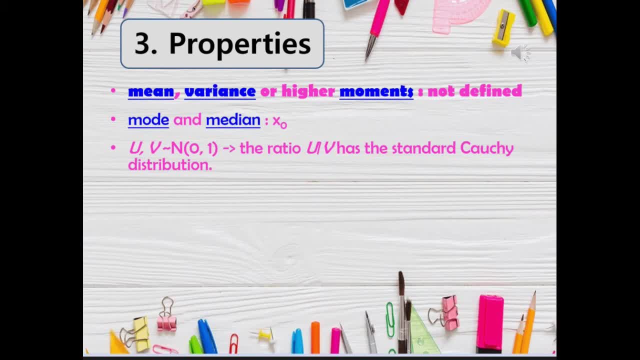 distributed random variables but expected value 0 and variance 1, then the ratio U over V as a standard Cauchy distribution, if X is equal to lambda e, raised to the power negative lambda X, simplifying that one, the area will just be equal to 1 over the mean. 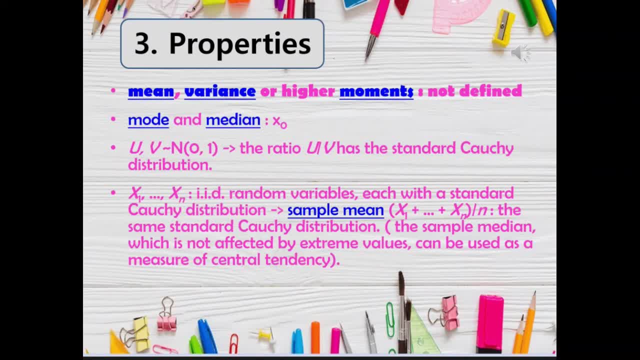 X sub 1 to X of N, our independent and identical distributed random variables, each with a standard Cauchy distribution. then the sample mean X sub 1 plus X sub n over n as the same standard Cauchy distribution, the same standard Cauchy. 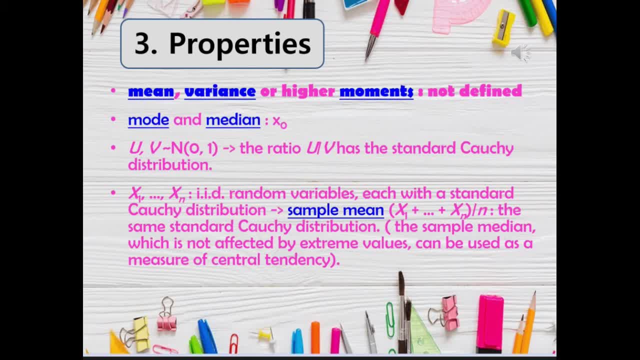 distribution. we have the sample median, which is not affected by the extreme values of our Linkedined- Durabil 2018 manual, can be used as a measure of central tendency. the standard Cauchy distribution is t1 and the characteristic function states that let x be defined. the Cauchy distributed random variable. 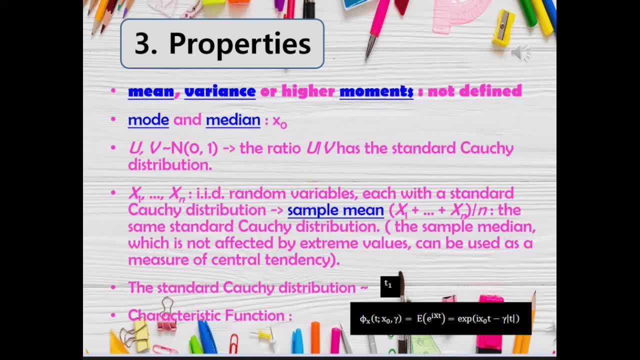 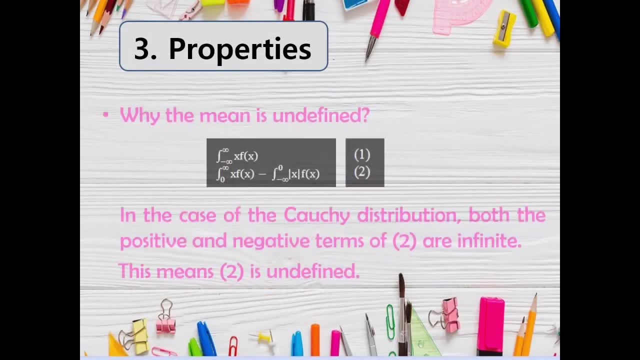 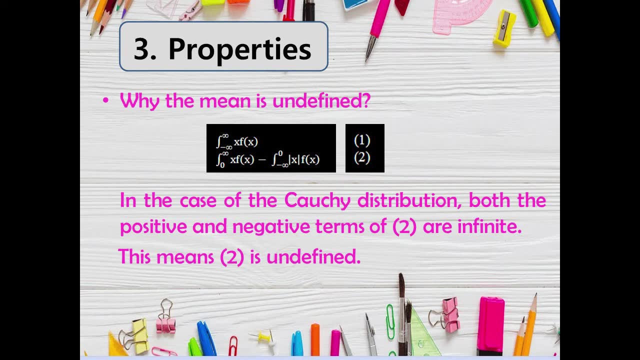 and the characteristic function of the Cauchy distribution is given by the formula given. one of the properties of the Cauchy distribution is that the mean here is undefined. now, why is the mean undefined? i have re read from wikipediaorg that if a probability distribution has a density function, f, then the mean, if it exists, is given by. 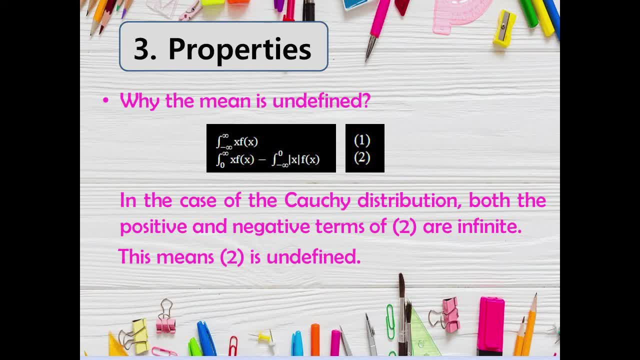 the integral, from negative infinity to positive infinity, of x times f of x, dx. we may evaluate this two-sided improper integral by computing the sum of two one-sided improper itten. parte qu appearing is t- t. you can now see that the one-sided improper integral of t is now: 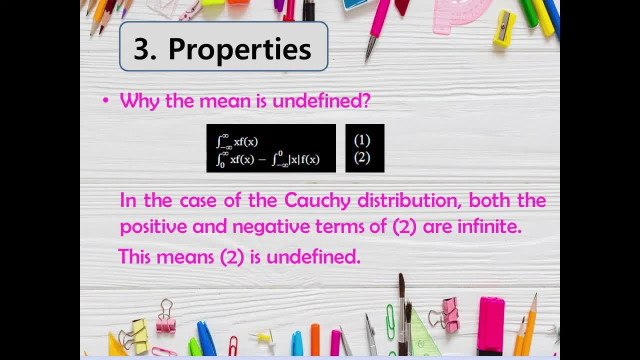 given as the one-sided one-sided integral in heli, or you can now see that the one-sided improper integral, And that is the integral from a to positive infinity of x times f of x dx, plus the integral from negative infinity to a of x times f of x dx for an arbitrary real number, a. 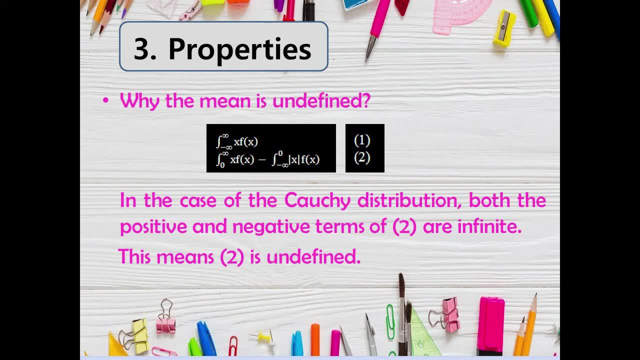 So for the integral to exist, even as an infinite value, at least one of the terms in this sum should be finite, or both should be infinite and have the same sign. But in the case of the Cauchy distribution, both the terms in this sum are infinite and have opposite sign. 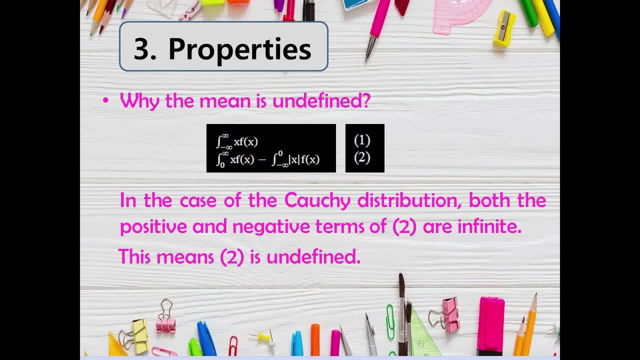 Hence it is undefined, and thus so is the mean. Basically, as Per Bell Amadio, the mean of any random variable is the integral with respect to x over the support of the variable of the function x times f of x, where f of x is the variable's probability density function. 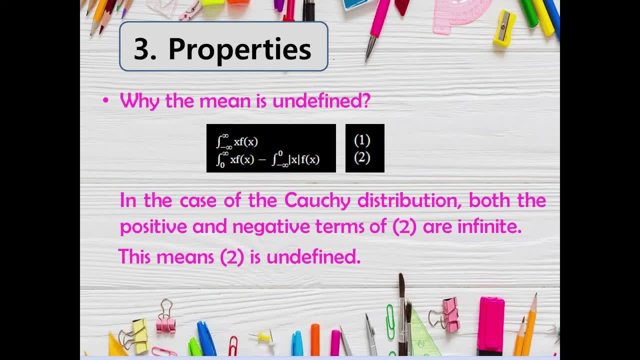 For the Cauchy. this integral is undefined. The support of a Cauchy random variable is minus infinity to plus infinity, So the integral is undefined. The integral representing the mean is an improper integral. The limit of the definite integral: x times f of x as the limits of the integration approach: minus infinity and plus infinity. 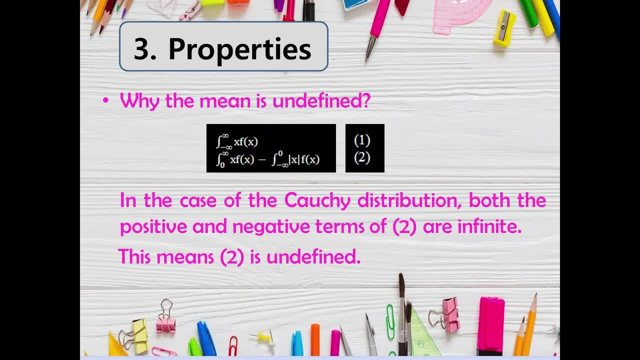 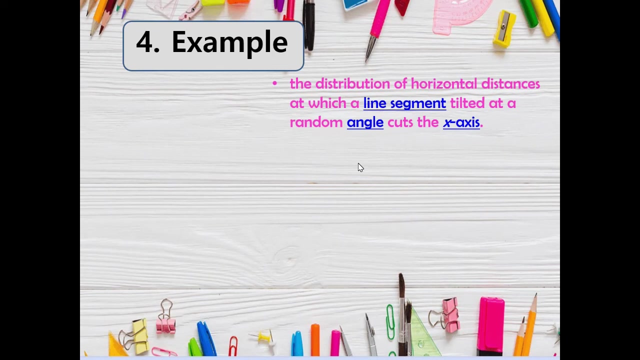 The tails of the Cauchy density function are heavy. They approach the x-axis more slowly than, say, the tails of a normal density And, as a result, the limits for the improper integral described are not the same. The integral for this integral is equal to x over b. 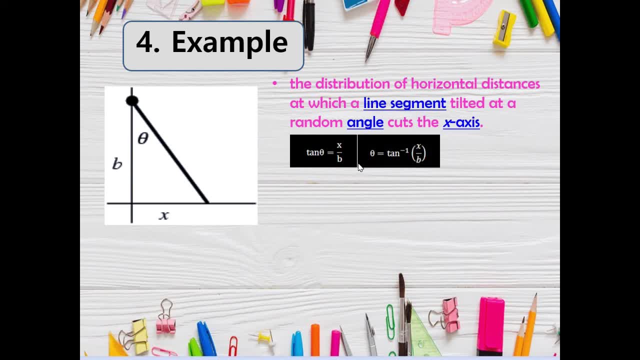 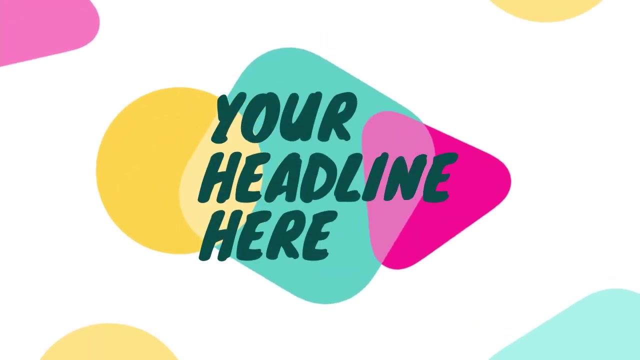 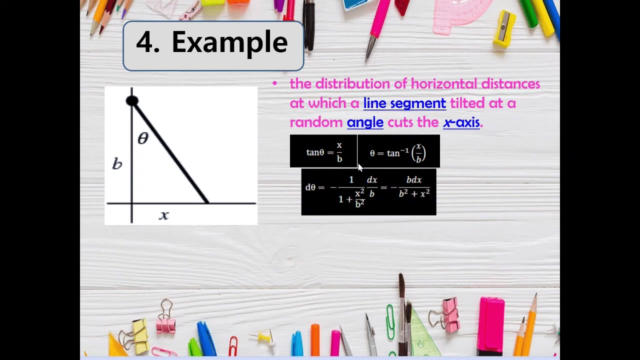 Then to derive the formula: theta is equal to tangent raised to the power of negative 1, which is the of tangent theta times the x over b d theta is equal to negative 1 over 1, plus x squared over b times dx over b is equal to negative b. dx over b squared plus x squared d theta.